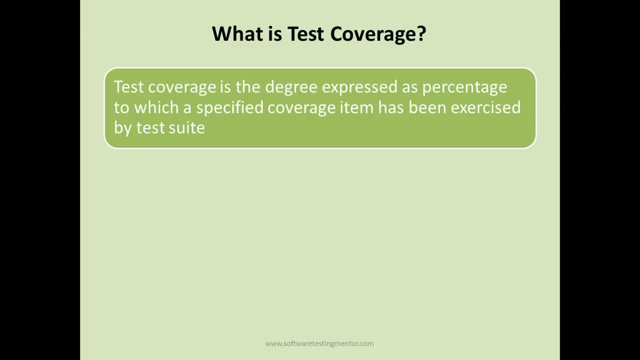 is the degree expressed as percentage to which I specified coverage item has been exercised by test suite. so, for example, if you are doing, if you have a certain set of requirements, then how, how much percentage of those requirements has been covered by the number of test cases that you have executed. so that's that, that calculated as a 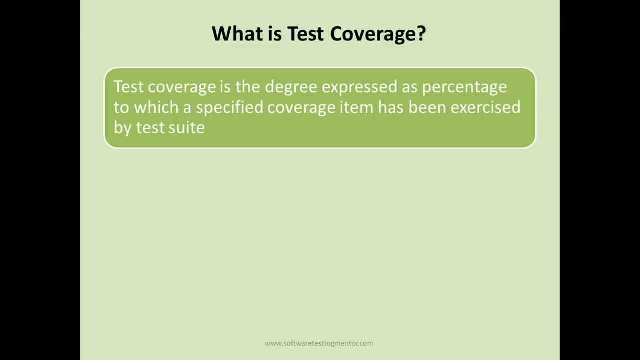 percentage is known as test coverage, so it's a degree expressed as percentage to which specified coverage item has been exercised by test suite. so the coverage, the formula to calculate coverage, is number of coverage items exercised divided by total number of coverage items into 100, so that's. 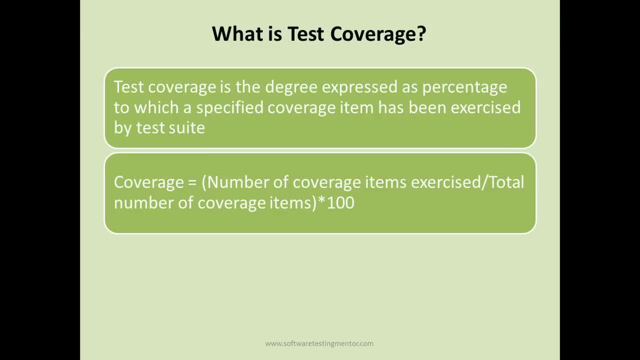 the formula to calculate coverage. so whatever numbers of the number of the coverage items have been exercised till now, and suppose the total coverage items are hundred, you have hundred and the requirements that have been tested exercised till now are, say, 80. so 80 by hundred into 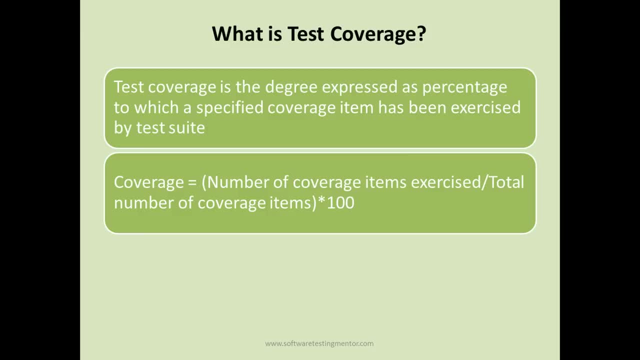 hundred, so eighty percent coverage has been done. then hundred percent coverage does not mean hundred percent tested, because coverage techniques measure only one dimension of multiple dimensions. so there are multiple dimensions of coverage. so hundred percent coverage of one dimension doesn't mean that your software is hundred percent tested. for example, hundred percent coverage of requirements. 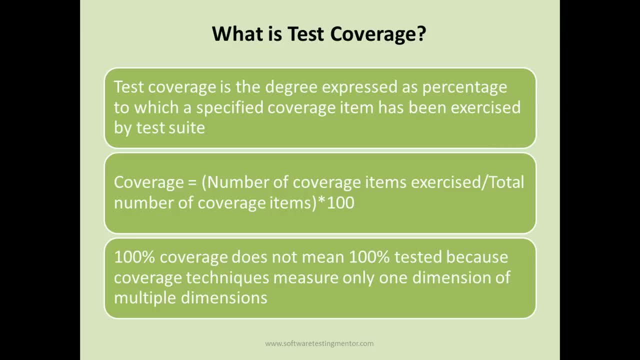 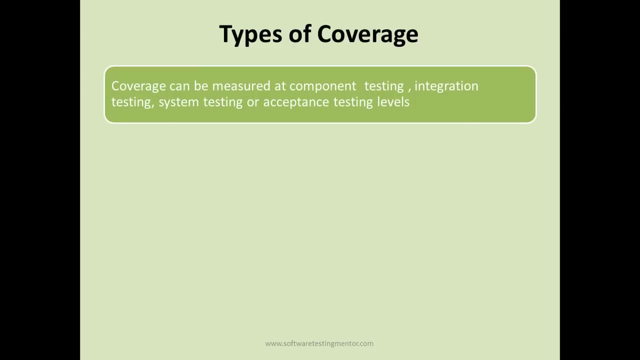 doesn't mean your software is hundred percent tested, because there are in many non-functional testing that needs to be done as well. there are many aspects of software testing. so what are the types of coverage? so coverage can be measured at component testing, integration testing, system testing or acceptance testing level. 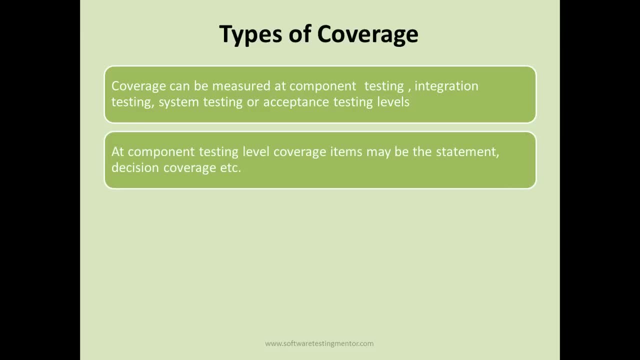 it can be measured at any test level. then at component testing level, coverage items may be the statement or decision coverage. so at component or unit level, your coverage item may be statement or decision coverage. at integration level, the coverage items are the interfaces or interactions with other software or system. and at acceptance testing level, coverage items may be requirements. 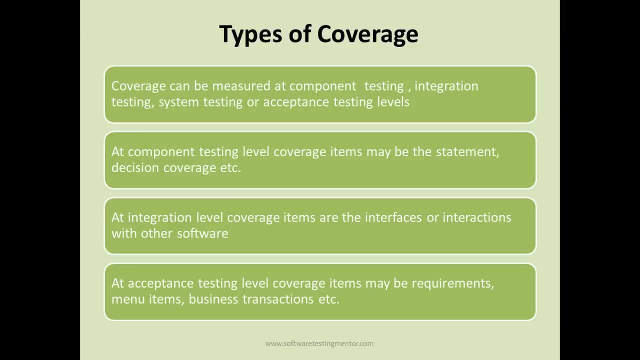 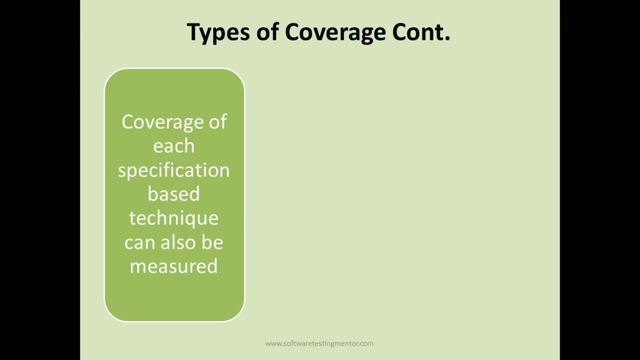 menu items or business transactions or end user scenarios. so what are the other types of coverage? so coverage of each specification based technique can also be measured. so, for example, you have some other, uh, some specification based techniques, for example, equivalence, partitioning, boundary value analysis, decision table. so what are the types of coverage for those so like? 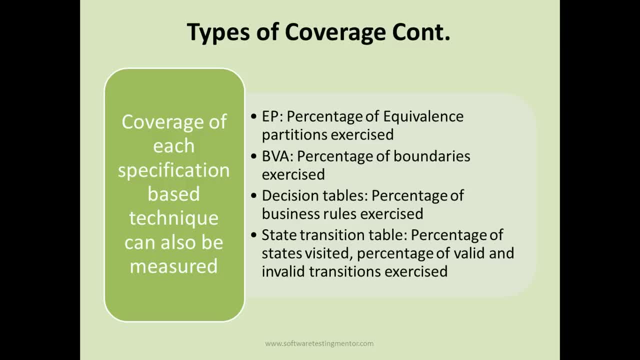 equivalence partitioning. percentage of equivalence partition exercised for boundary value analysis. percentage of boundaries exercised. then for decision tables, percentage of business rules that have been covered or completed by the test cases. then is in state transition table, the percentage of states visited. percentage of valid and invalid transitions exercised by the test suite. 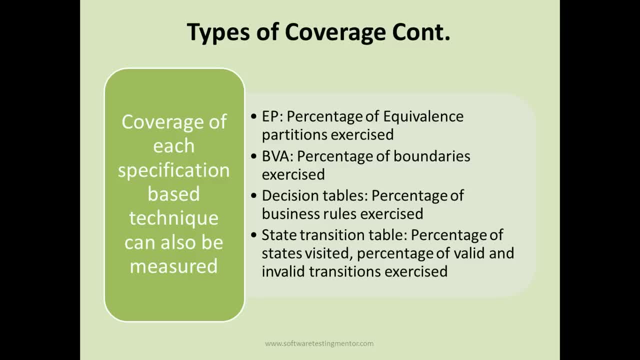 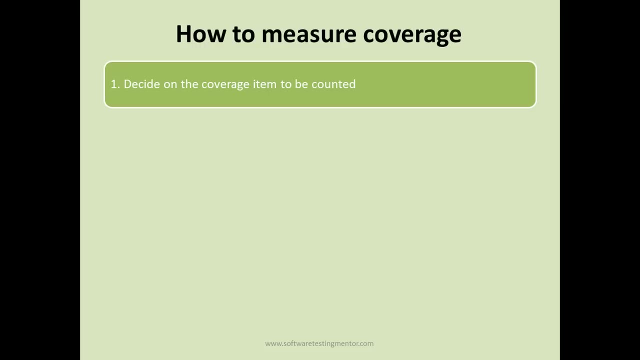 by the number of test cases that you have executed. so these are some of the coverage of each specification technique that you can measure. so how to measure the coverage? so the first step is to decide on the coverage item to be counted. so first thing is to decide what you want to count, what is the 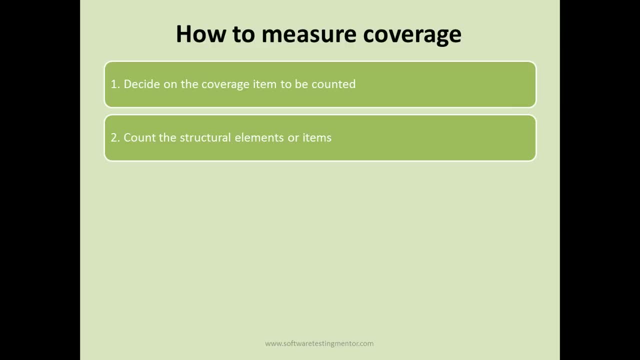 coverage that you are going to measure. now. the best way to do that is to calculate the item that you want to count. the second thing is to count the structural elements or items. the second thing is you need to count the structure element, all the items that needs to be covered, so that total calculation, total count of 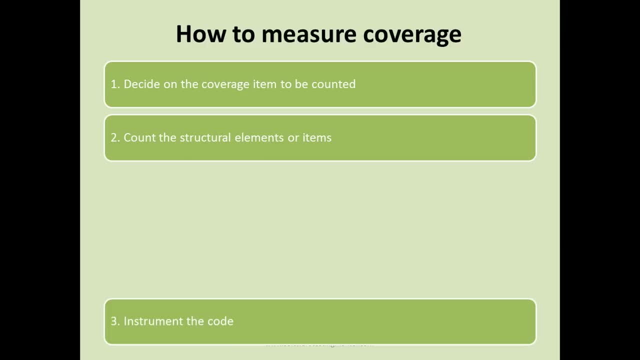 the coverage items need to be there in the first place. then you need to instrument the code. so basically in in white box, testing your code coverage or the coverage measure is mostly done by the tools. so tools are intrusive in nature and you can instrument the code in order to find the coverage of. 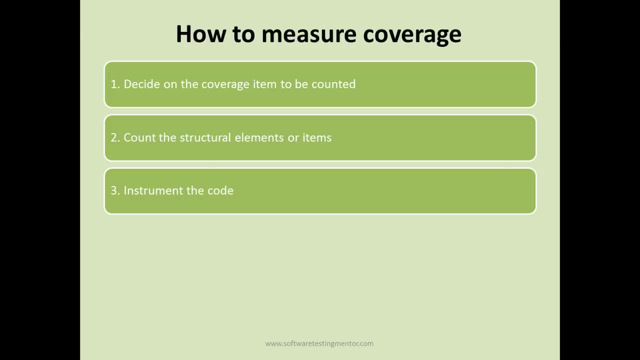 elements or items. so third step is to instrument the code and then you run the tests for which the coverage measurement is required. so you run the test against the instrumented code for for which you require the coverage measurement and finally, using the output from the instrumentation, you determine the percentage of items that have been. 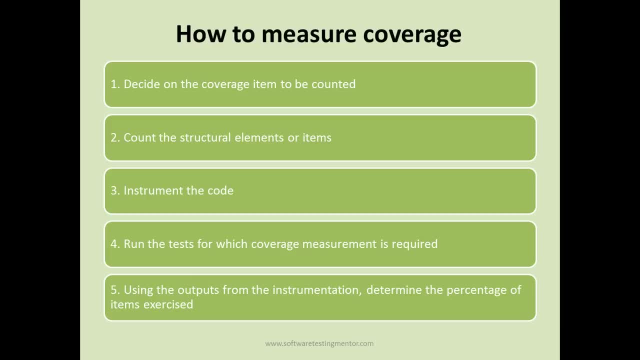 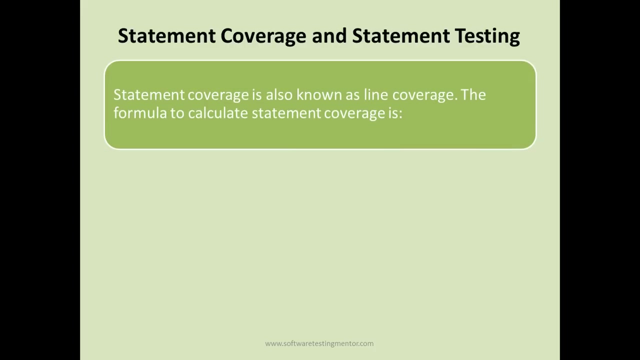 exercised. so these are simple steps that are done to measure the coverage of items. so what is statement coverage and statement testing? so statement coverage is also known as line coverage. the formula to calculate statement coverage is: statement coverage is equal to number of statements exercised upon total number of statements in 200. formula is pretty simple. it's similar to: 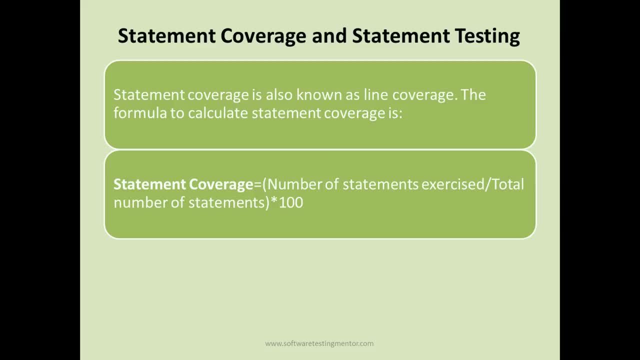 coverage, the generic formula. so statement coverage is also known as line coverage. it is basically the coverage of the number of statements in the code when you you the number of statements of code exercised when you execute your test suite. so suppose your test suite has a hundred test cases once you execute all. 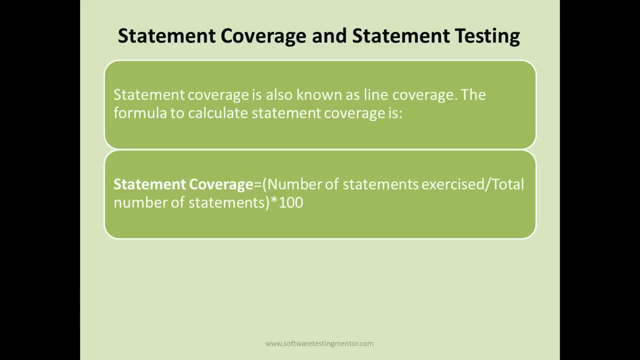 those hundred test cases. how many line of codes have been affected by executing those hundred test cases? that's known as statement coverage, and percentage of statement coverage can be calculated using the formula. then studies in software industry have shown that black box testing may actually achieve only 60% to 70% statement coverage. this leaves around 25. 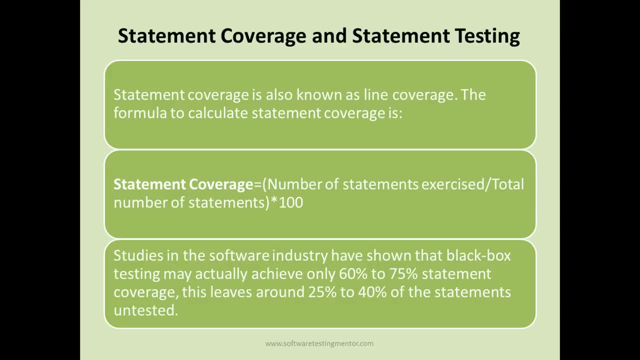 to 40 percent of the statements untested. so with black box techniques it has been seen that, whatsoever how I mean, it doesn't depend how effective your test cases are, the black box testing test cases are. it has always been seen that a the the number of number of the statement coverage is not always hundred. 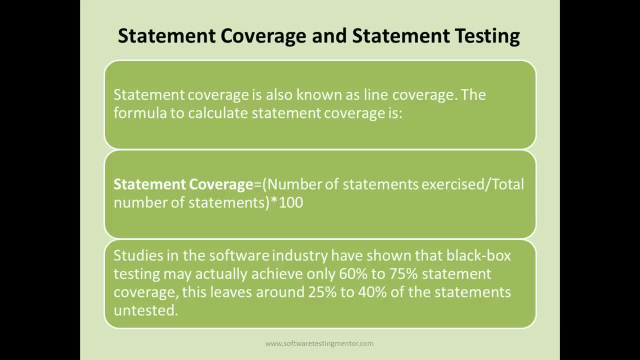 percent it's. it's much less than that in black box test design technique. so that is why requirement for statement coverage and statement testing is there, and that is why you need to do white box testing, yeah, along with the black box test techniques. so let's take an example of statement coverage to its 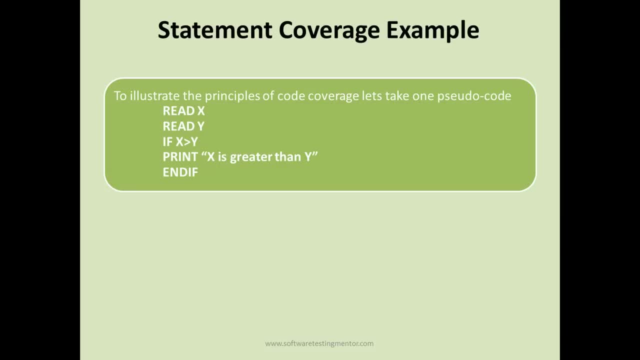 illustrate the principles of code coverage. I'll take just a simple pseudo code. it's not specific to any programming language and it's just a just a pseudo code, dummy code. so the code is: we are reading a value, then read X, read Y and then if X greater than Y, then we are printing a statement and 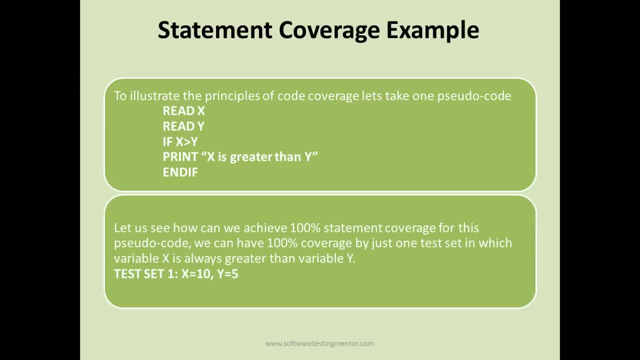 just ending. so in this case, let's see how we can achieve 100% statement coverage. so in this case, in this pseudo code, you can achieve 100% statement coverage with just one test case. so if you set X to 10 and Y to 5 or any any value of X greater than Y, all the statements will get. 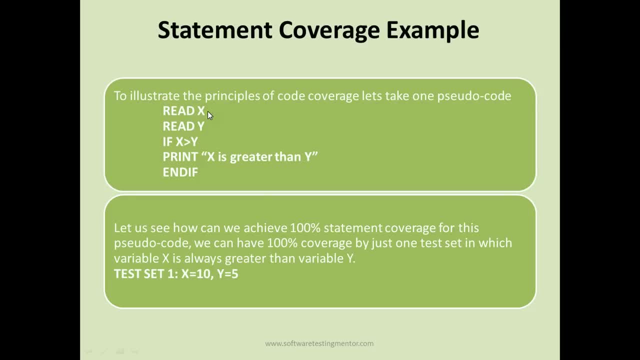 executed. so it will read a value for X, read value for Y. it will come to the this line. it will execute this line as well. then it will print X is greater than Y and then end. so all the lines of code will get exercised with just one test. 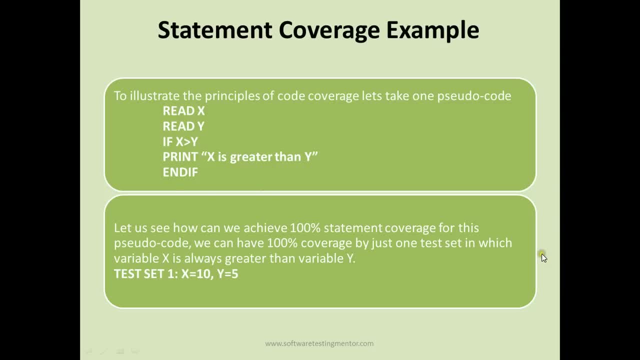 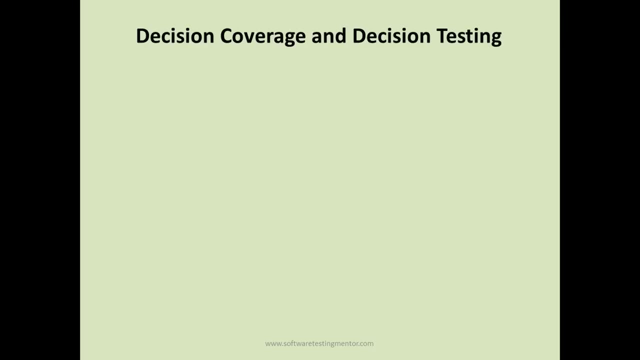 case, so you'll get 100% coverage, a statement coverage in this scenario, then what is decision coverage and decision testing? so, whenever there are two or more possible exits from the statement- for example, if statement do while or case statement- whenever there are two possible exits and you testing you, you test those decisions to because there are two. 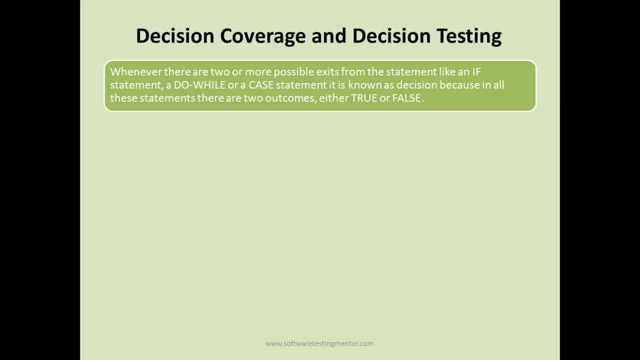 exists, the one is either true or false. so whenever you are testing these two outcomes, it is known as decision testing. so decision coverage ensures that each outcome that is true and false is of control statement- has been executed at least once. decision coverage ensures that your decision outcome- true and false- have been executed at least once. 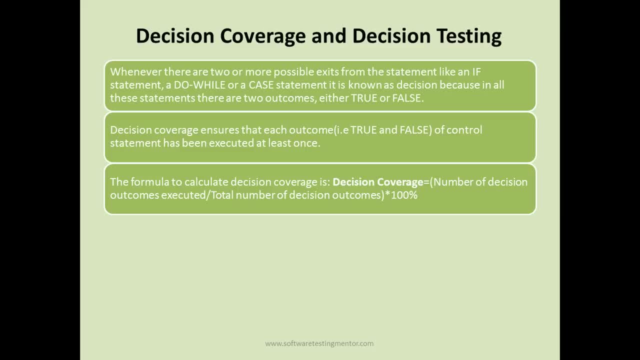 then the formula to calculate decision coverage is same number of decision outcomes that have been executed upon total number of decision outcomes in the software into hundred. so that's the formula to calculate decision coverage. and research in industries have shown that even if functional testing has been done, it only achieves 50 to 60 percent decision coverage. so black box testing. 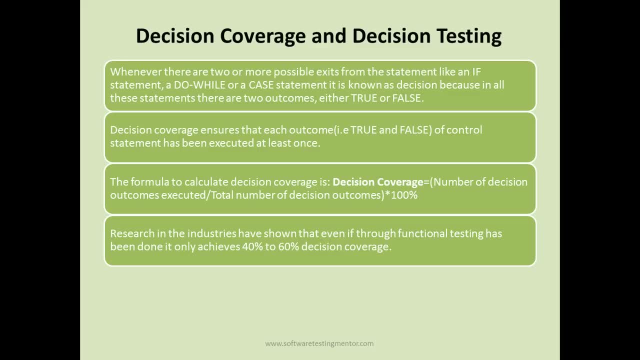 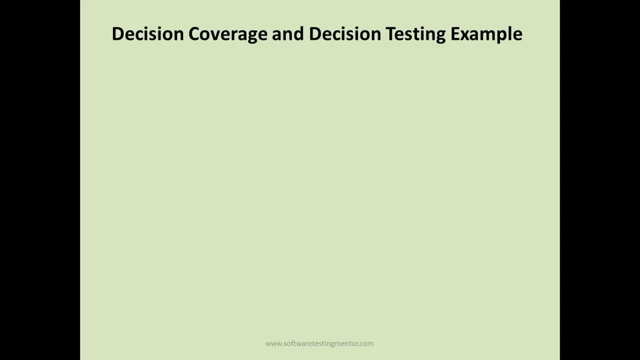 doesn't achieve 100 percent of decision coverage, then decision coverage is stronger than statement coverage and it requires more test cases to achieve 100 percent decision coverage. so decision coverage is stronger than statement coverage and you require more number of test cases to achieve 100 percent decision coverage. let's take an example. 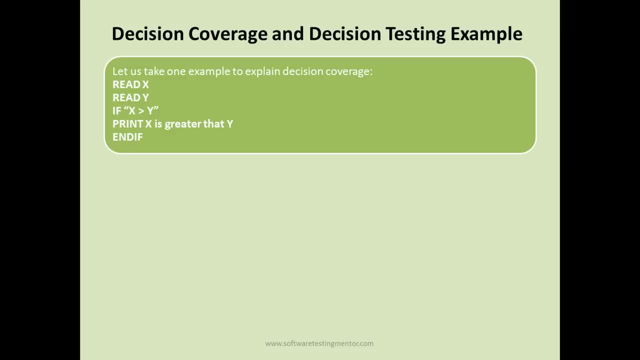 to understand decision coverage and decision testing. so we have taken the same pseudocode. you're reading two values. if X is greater than Y, we are printing and statement and then just ending so to get 100% of statement coverage. there was just one test case sufficient to exercise all the 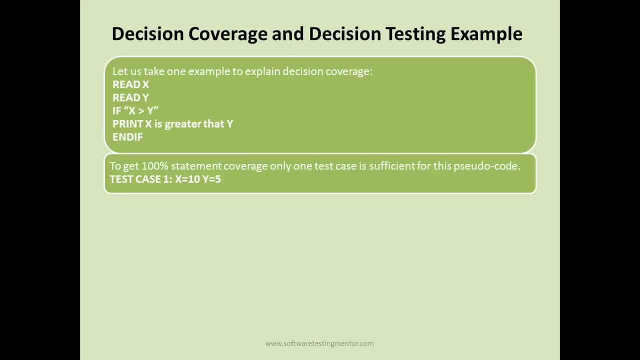 statements of this code. but in order to get a decision coverage, you won't be able to achieve this hundred percent decision coverage by this test case, because it it checks that X is greater than Y, which is true, and then it passes that. so only for the if condition only true decision has been exercised, and for 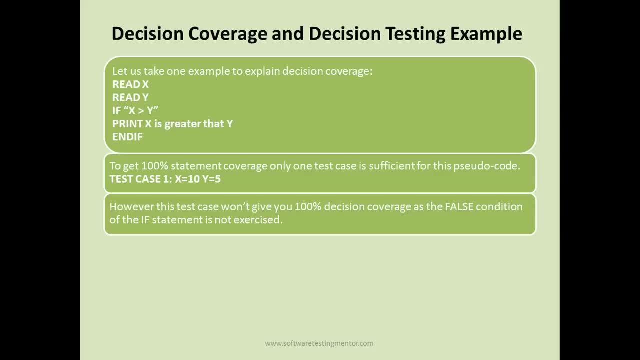 false has not been exercised. so in order to do hundred percent decision coverage, you need to exercise false condition as well. so for that you need a value of X which is less than Y. so the final test set for hundred percent decision coverage will be: there will be another test case in which value of X 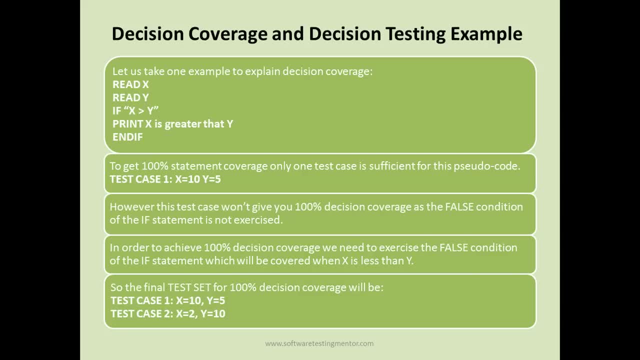 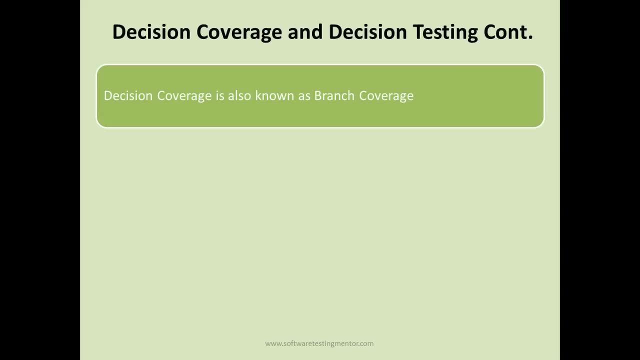 will be less than Y and then you will be able to achieve hundred percent decision coverage. so decision coverage is also known as branch coverage. then hundred percent decision coverage guarantees hundred percent statement coverage. but hundred percent statement coverage does not guarantee hundred percent decision coverage. so if hundred percent decision coverage is there, then 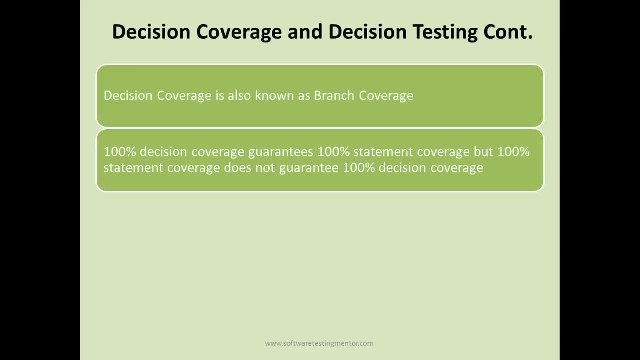 you can say hundred percent statement coverage has been done, but it's not true vice versa. decision coverage cannot test hundred percent of the software code. so these techniques are useful for specific types of tests. so the types of test techniques and combination test techniques should be chosen very wisely. 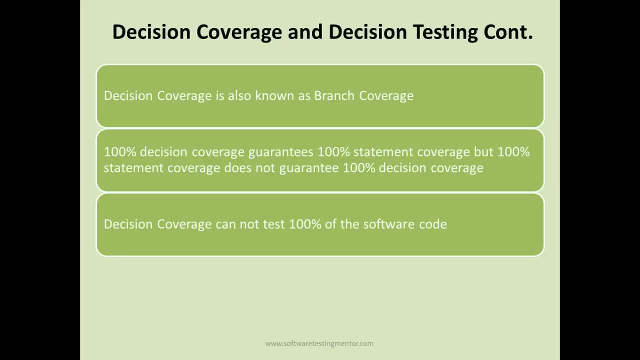 and mix and match of those test techniques should be done to achieve best possible test coverage or best possible testing. so decision coverage is not suitable for any complex decision items, for example the statement given if a is greater than B or a less than 10 and a plus B is equal to 20. so it's a complex decision item decision. 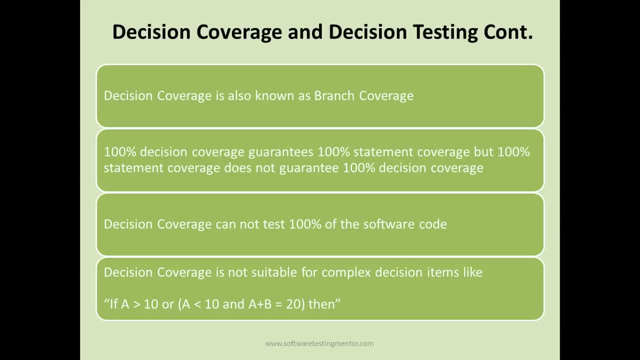 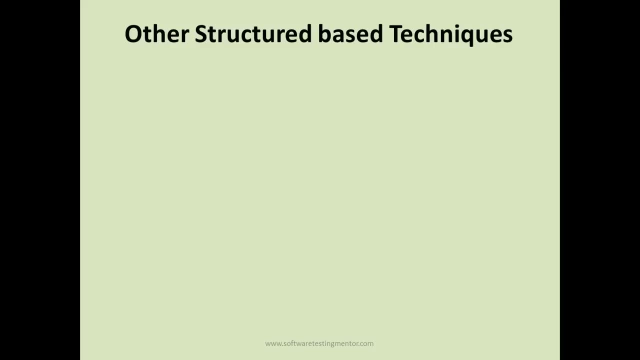 coverage or decision testing is not suitable for these kind of statements or items, so for for more complex items. so there, as per ISTQB syllabus, these are only two techniques that you need to know a bit in detail, and it should be able to identify the test cases based on. 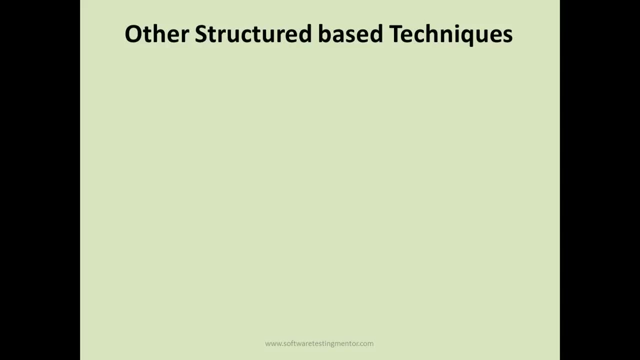 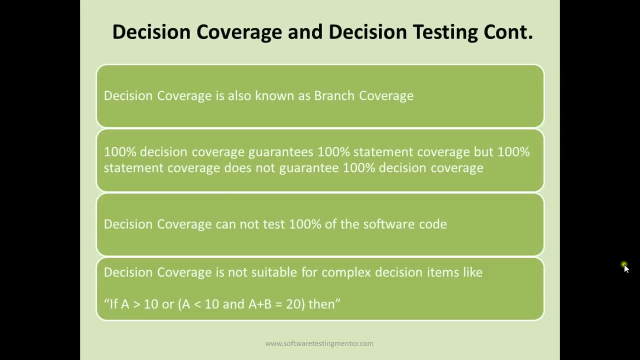 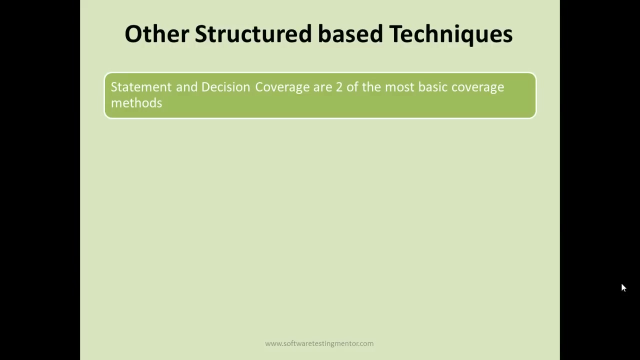 the pseudo code for these two techniques. and then for there, there are other structure based techniques, other complex structure based techniques which will help you to identify decision coverage for complex decision items, for example like this. so what are the other techniques? so statement decision coverage are two most basic coverage methods. other, more complex structure based.